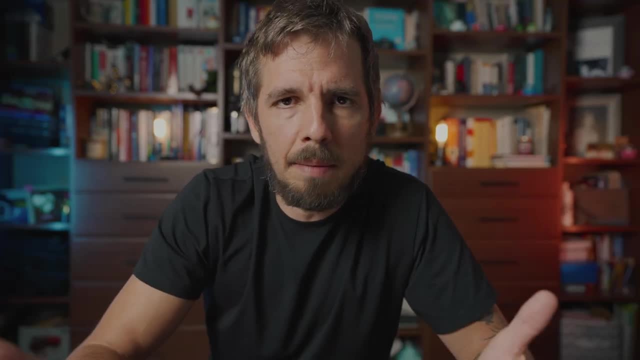 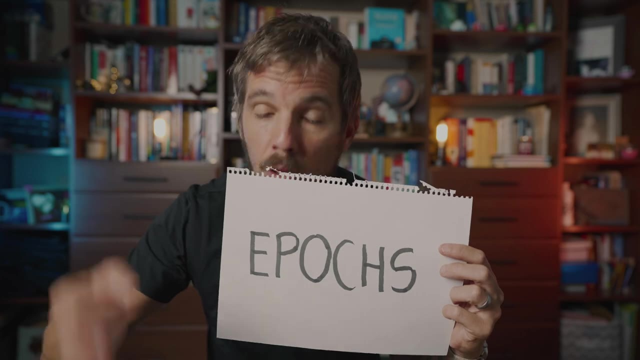 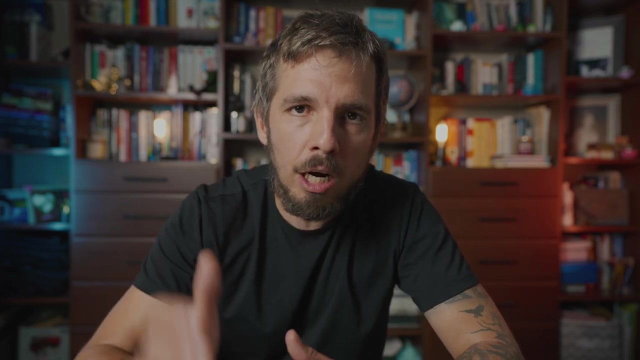 guess it's not necessarily time, but something similar. We call it the number of iterations or epochs. Train a model for too many epochs, and you'll underfit. Train it for a few epochs only, and you'll end up underfitting. But how do we find the perfect number of epochs to train a model? 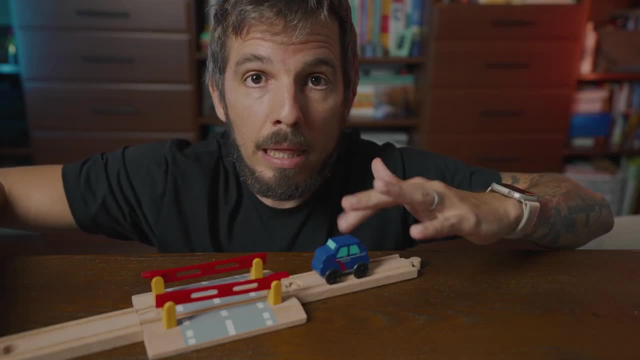 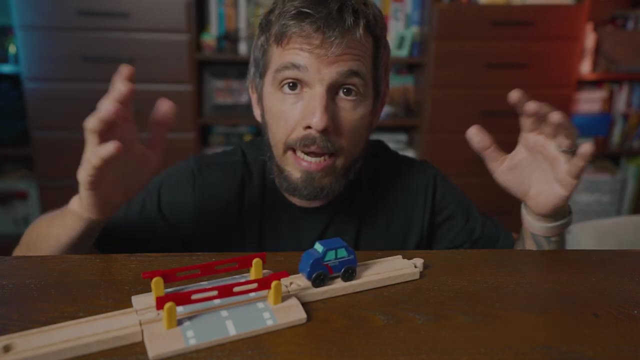 Let's play a dumb game here. This here is a police car. It's gonna start driving and I want it to stop between the barriers. It cannot stop too early and it cannot stop too late. It's gotta stop exactly between the barriers. Now, police cars. 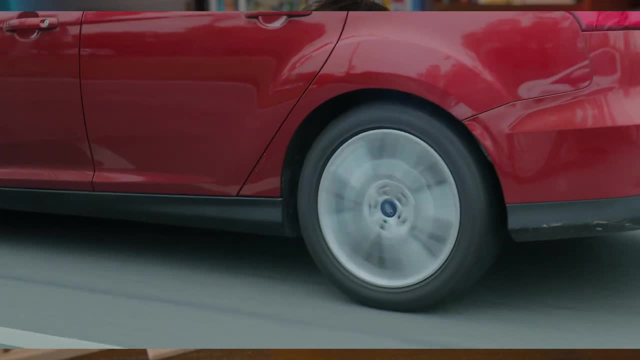 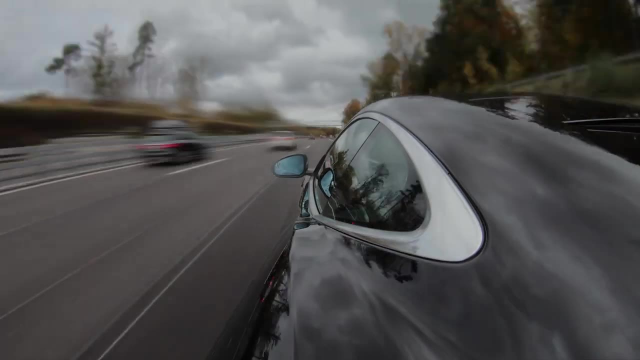 have brakes, so this should be pretty simple. The only thing the driver needs to do is to push the brakes exactly at the right time, And that's exactly what we need to do with our model. The car knows when to brake because it sees the red barriers, But how do we know? How do we know? 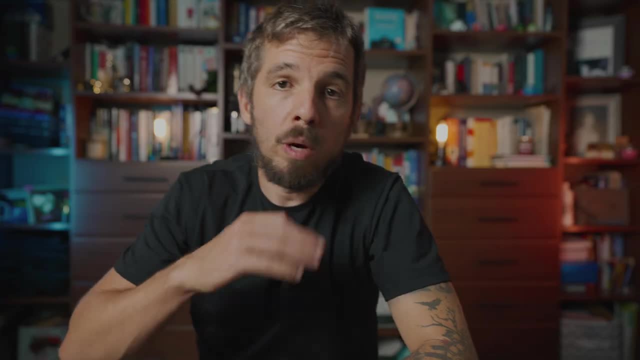 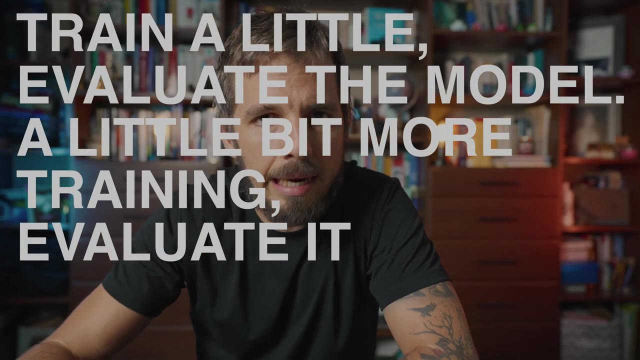 when is the perfect time to stop our training process? We need a way to evaluate our model as we train it. Train a little, evaluate the model a little bit more training, evaluate it again. This way, we can see how the model is doing. 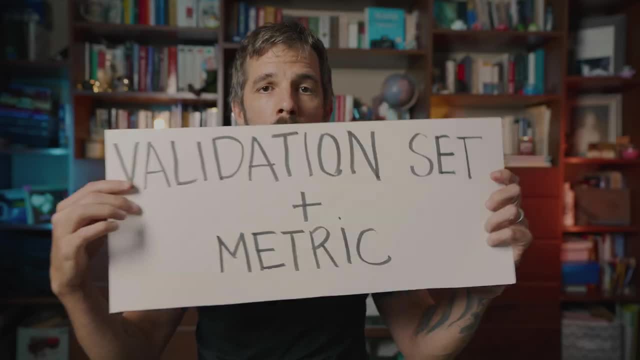 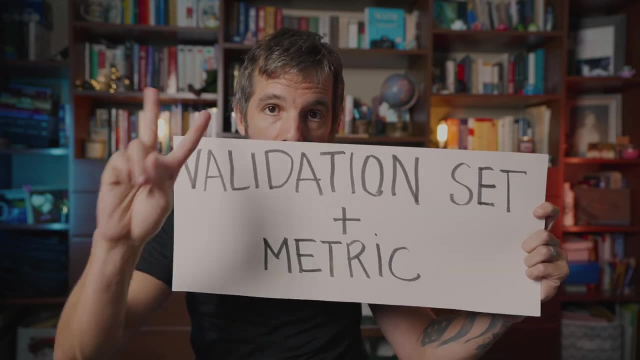 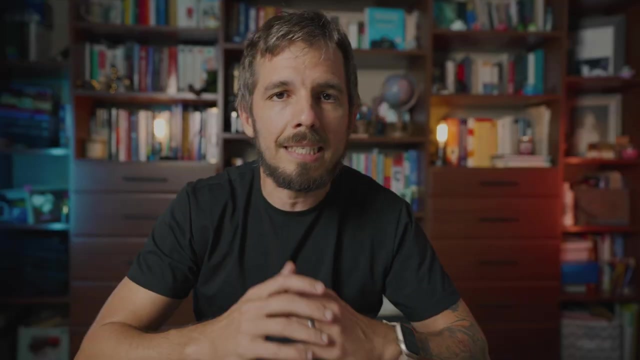 in real time. To make this happen, we need two things: Number one, a separate holdout set that we call a validation set. That's where we will evaluate our model. And number two, a metric that measures the performance of the model. That's it. I'm sure you've done this. 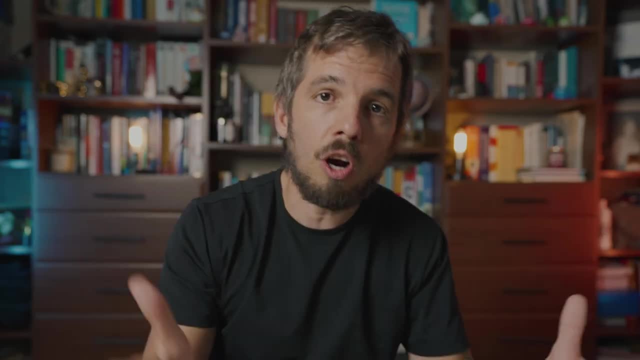 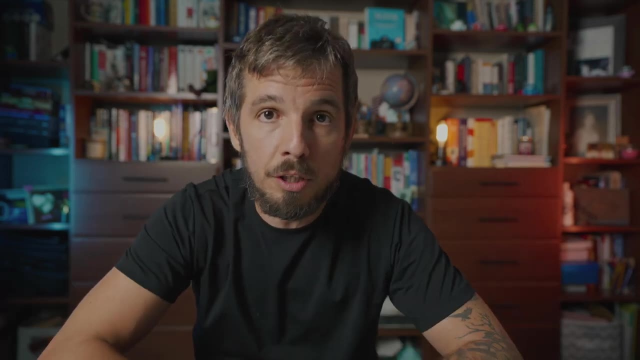 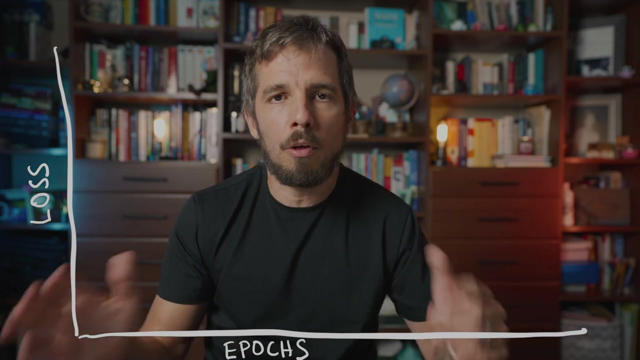 one million times before. With these two, we can start training our model, evaluate it after each epoch and start plotting our metric to see how the model is doing. Now look at the chart on the screen. Assume that we pick the validation loss as the metric to measure how the model is. 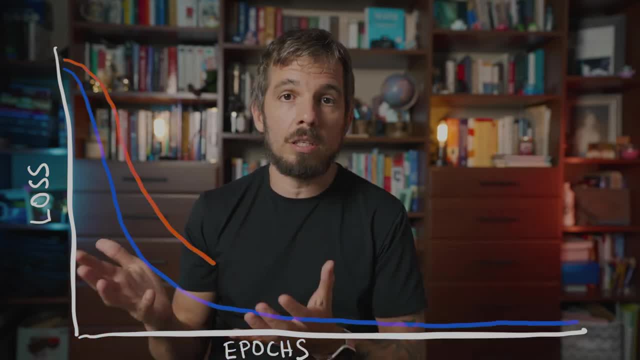 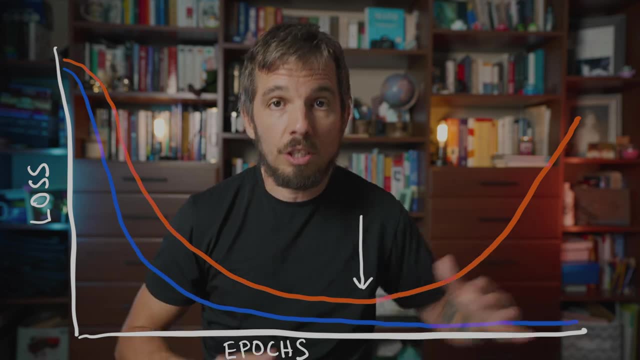 doing. The blue line is the training loss, while the orange line is that validation loss, And I want you to notice what happens around this area here: Suddenly, the validation loss starts increasing, indicating that our model is getting worse If you train for too long. that's exactly. 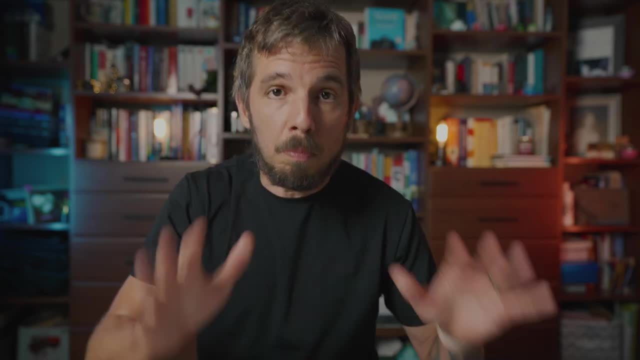 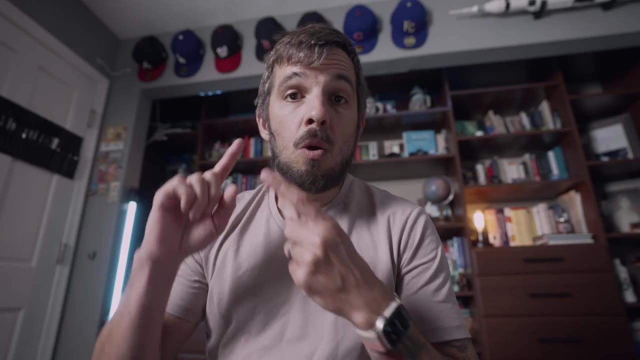 what you'll see, And that's it. That's the point where we want to push the brakes and hold the training process. There is a problem with this: If you train for too long, you will lose your model. There is a lot of manual work in it. We have to train longer than necessary to find the 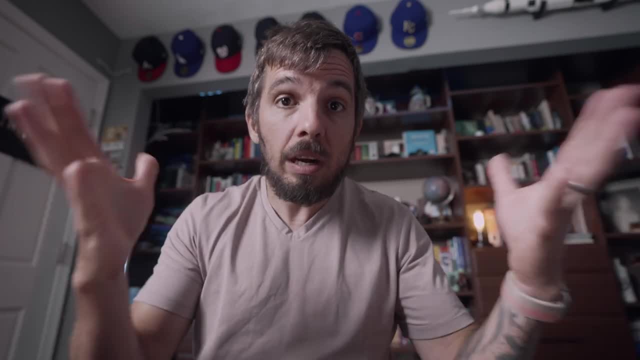 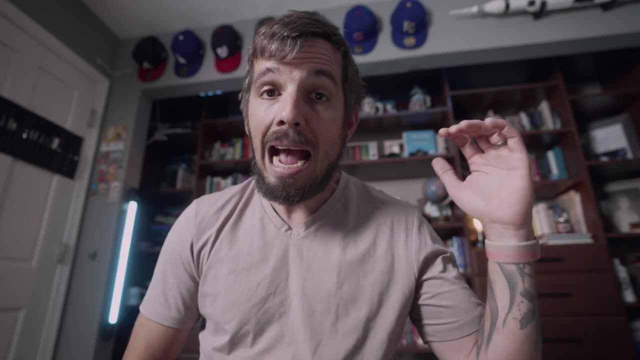 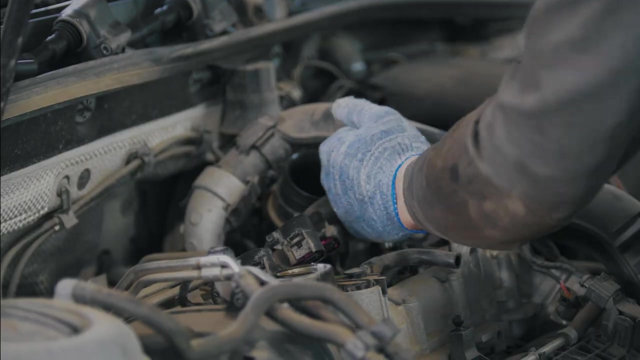 inflection point. We have to draw a chart and look at it to decide when to stop the process. And then, when we do, we must retrain the model from the start And, most importantly, if we change anything, anything at all, with our model, we must restart the whole process. 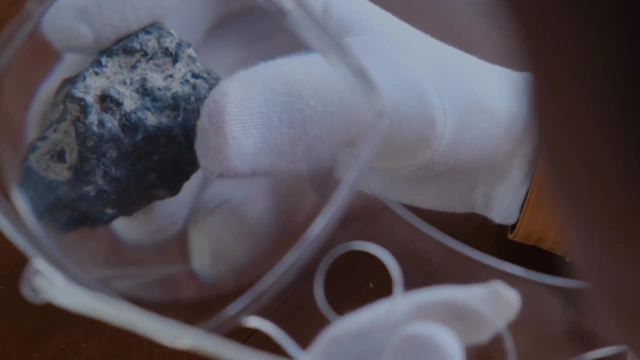 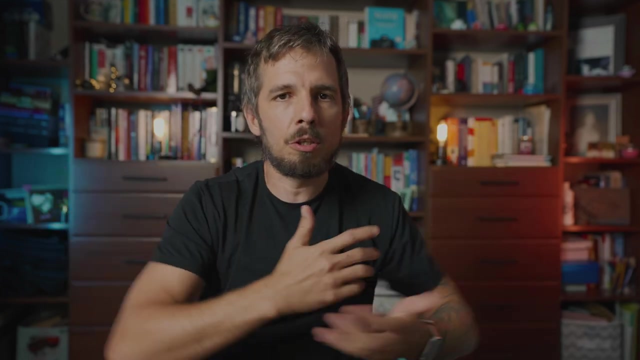 from the beginning to find a good number of epochs. again, Manual work Not good, So let's make it better First. no shorts. We don't want to be looking at anything to make any decisions. We want that to happen automatically. But how do we do that? 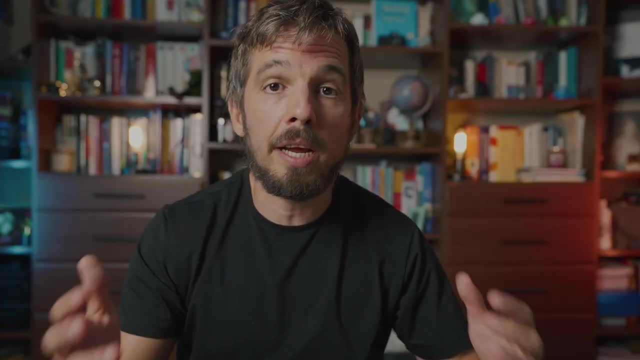 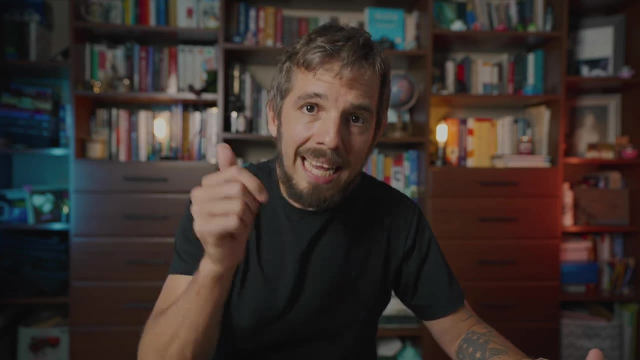 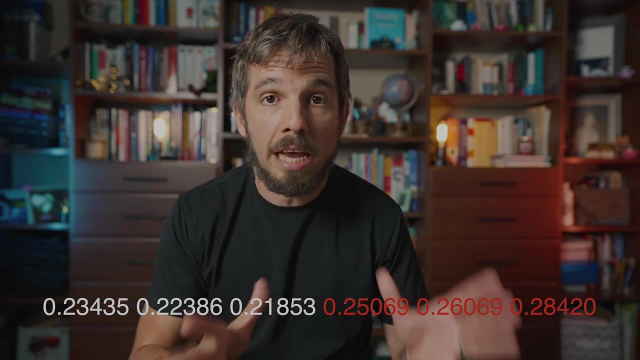 Well, think about the validation loss. For the best part of the training process the validation loss decreases until it hits that inflection point. when it increases, We can detect that automatically. If we watch the loss value and notice that the direction changes for a few consecutive epochs, we can assume that's the point of no return. 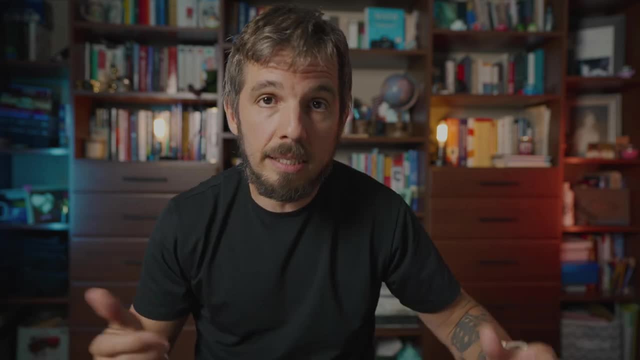 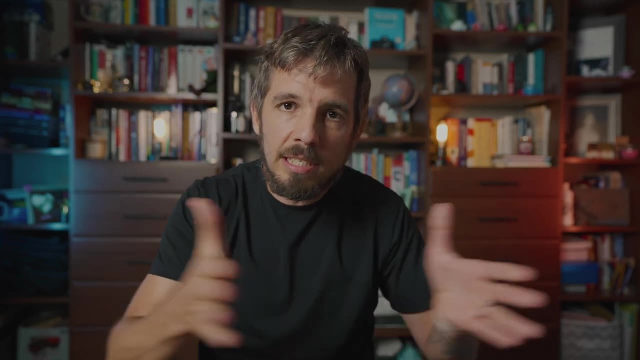 And hold the training process. If there is a lot of noise in the training process, we might see the validation loss oscillating up and down. We need to give it time to show a consistent pattern for a few consecutive epochs. We call that patience. Secondly, 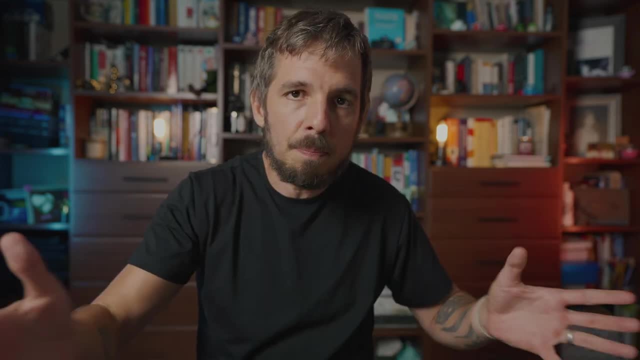 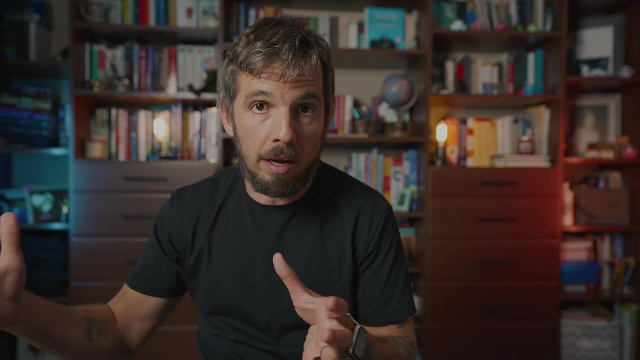 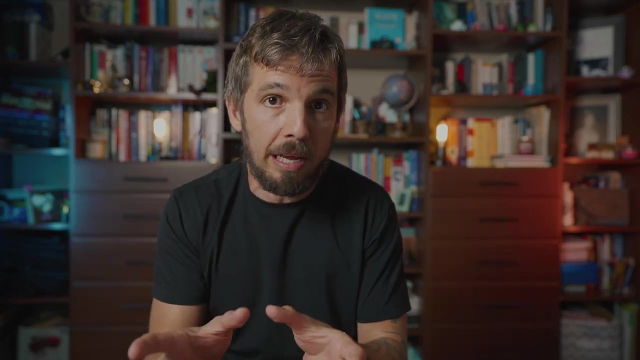 since we need to wait for a few consecutive epochs before stopping the process. by the time we make that decision, the model has been overfitting for a while, So we need to find a way to get time and grab the model before it started overfitting. This is how we solve the problem. As we train the model, we want to store a copy of the weights, as long as the validation loss of that copy is better than the previous one that we saved. That way, as soon as we stop the training process, we will have the best set of weights ready and waiting for us. 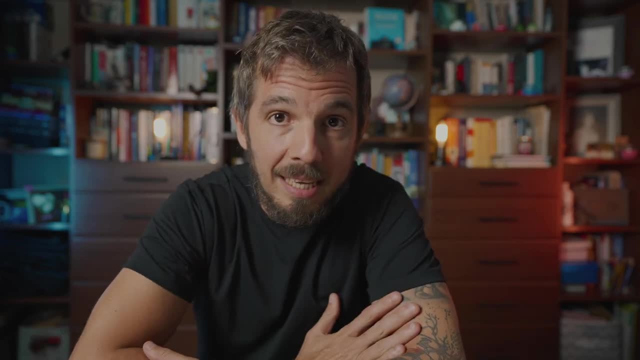 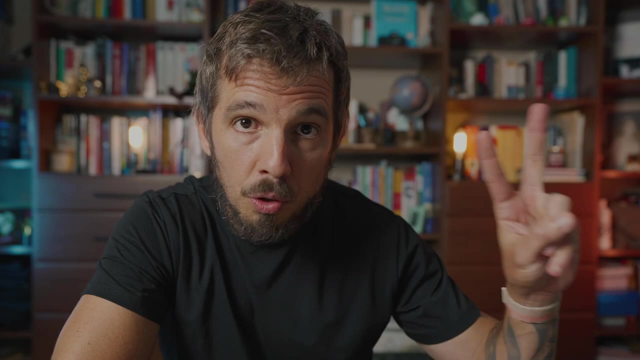 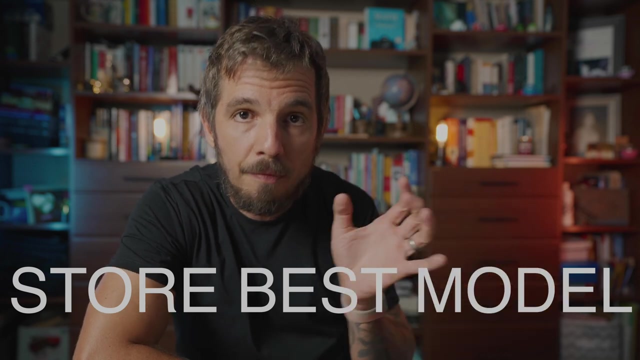 And that's every ingredient we need. We call this process early stopping. The four components of early stopping: Number one: a validation set. Number two: a metric to measure the model's performance. Number three: the ability to save the best copy of our model as we make progress. 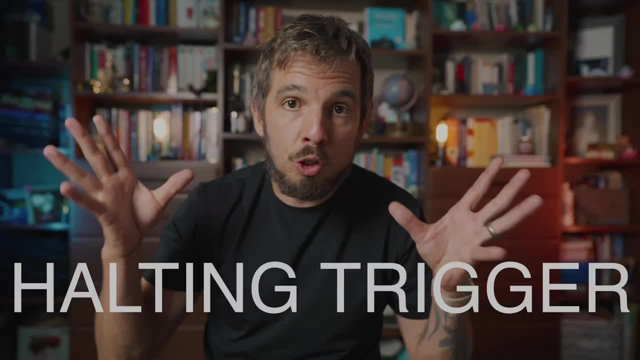 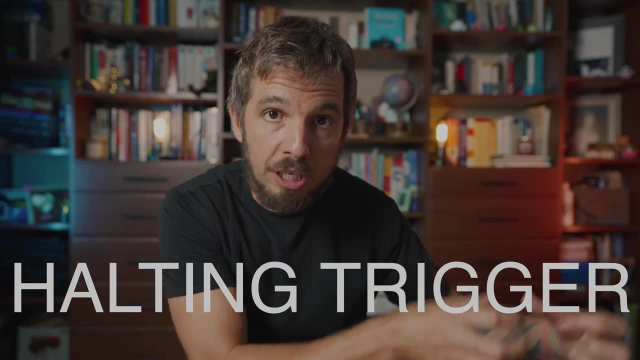 in the training process. And finally, number four, a trigger that halts the training process as soon as we notice that the metric we picked has been going in the wrong direction for a few consecutive epochs. That's it. Every major library out there supports.